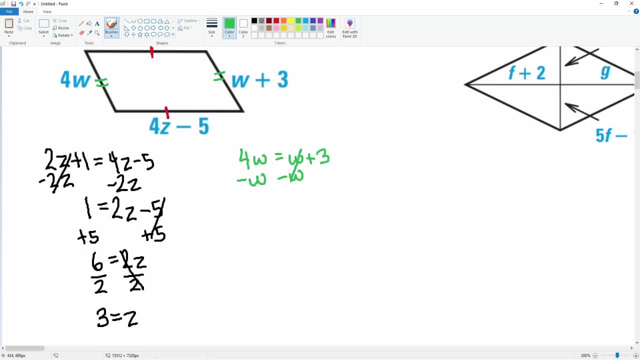 w to both sides, w and the w on the right does cancel. 4w minus w is 3w equals to the 3 on the right Divide by 3. to both sides. 3 over 3 does cancel, leaving you with just a. w is equal to 3 divided by 3.. It is 1.. So z is 3.. w is 1.. Those are the. 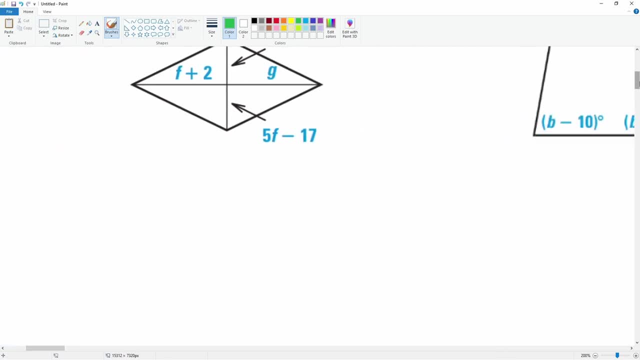 variables that we are looking for Next. Okay, we have this. Okay, Now we know that the diagonals are bisect. So this going to be the same as this: because the diagonal is bisect, then we know that this diagonal, which? 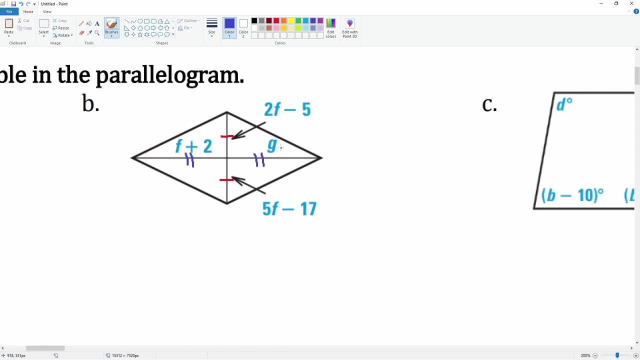 is left to right bisects as well. okay, so that gives us our two parts. all right, i'm going to. i'm going to solve for my f first. so 2f minus 5 is equal to 5f minus 17. okay, i'm going to subtract. 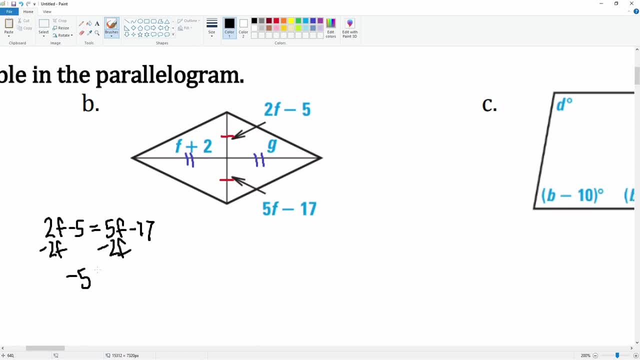 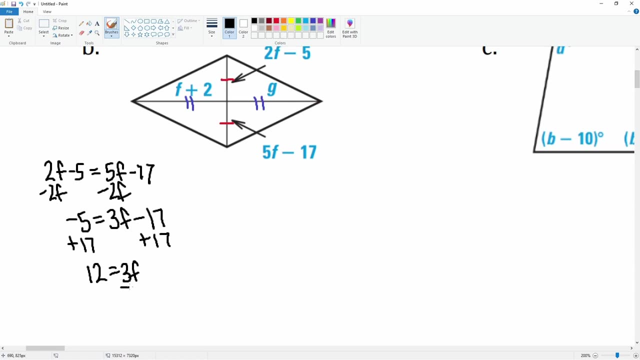 2f to both sides, leaving you with a minus 5 equals to 3f. minus 17 plus 17 to both sides. this gets you a 12 is equal to 3f. then you want to divide by 3 to both sides: 3 divided by 3 is just f. then you have 12 divided by 3, which is 4. 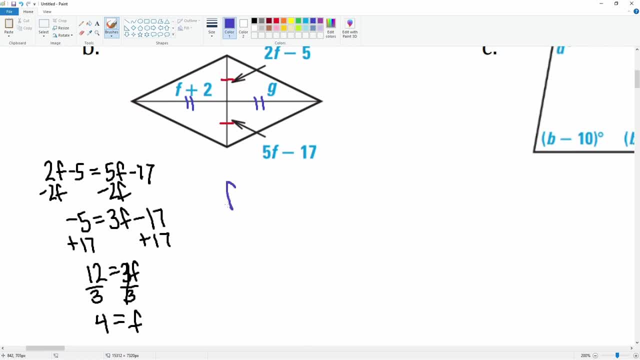 the next equation. it is the blue part. so that's the f plus 5f minus 5 is equal to 3f minus 17 plus 17 to both sides. this gets you a. 12 is equal to 3f plus 2 is equal to the g. we know what the f is. the f that we solved for from before was 4. 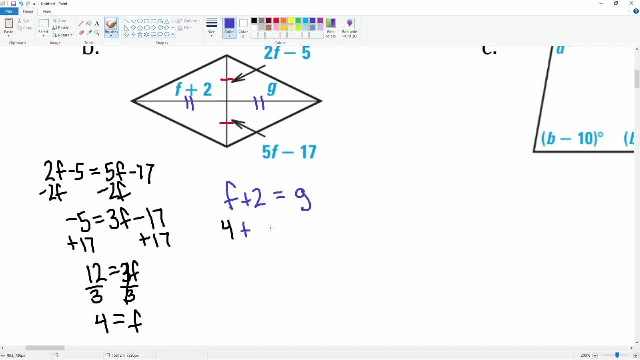 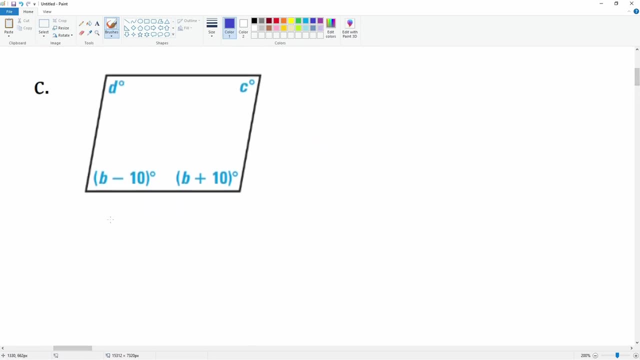 so we can substitute that in. okay, then we have: plus 2 is equal to g, 4 plus 2 is 6, that equals to g. okay, this equation required us to solve for f first, then substitute it in next. let's see for c. okay, we know that, the angles here. we know that. 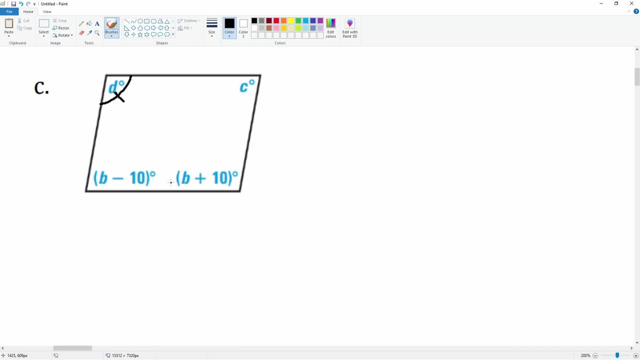 this angle is congruent to this angle, so we could set those two equal to each other, but that's going to be useless, because do we have two different variables? then we have. this is congruent to this, i just don't want to cover it. okay, that's useless because the these two have two different.